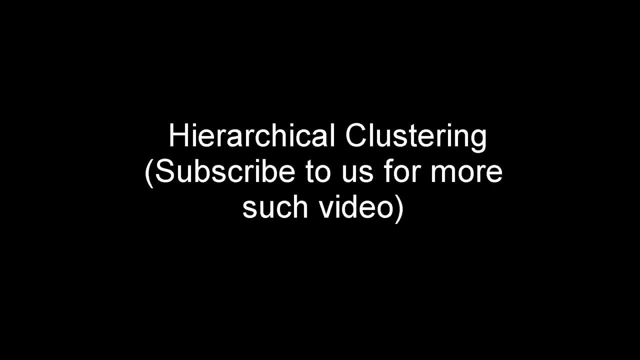 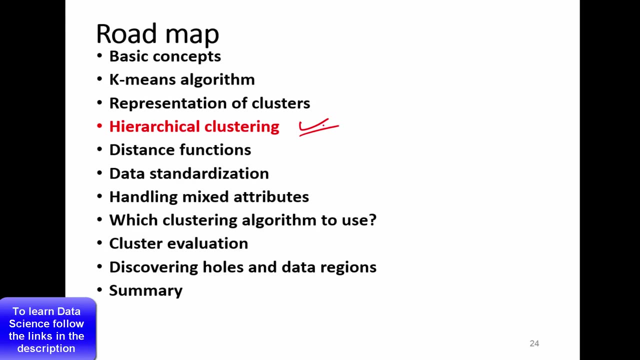 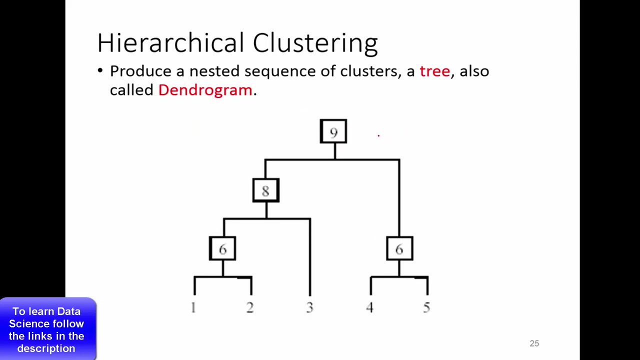 The next thing that we'll study is hierarchical clustering. Philosophically it's different from K-means clustering. It looks much better when explained with the help of a graph or a tree, rather, and we call that as a dendrogram, And we'll try to understand how we build this. 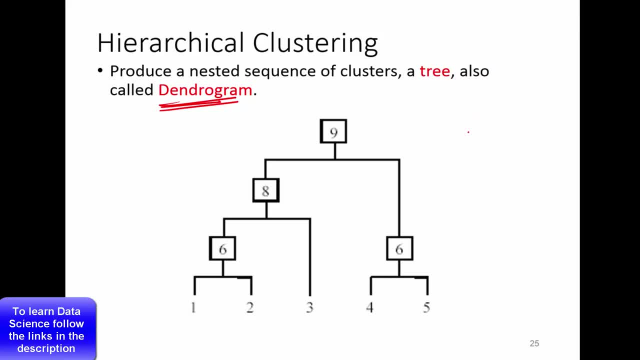 dendrogram because there are few steps involved and then we'll see how it actually helps on understanding how many clusters we have and what the clusters are. So we don't have to provide explicitly how many clusters. you know the value of K, the way we used to do. 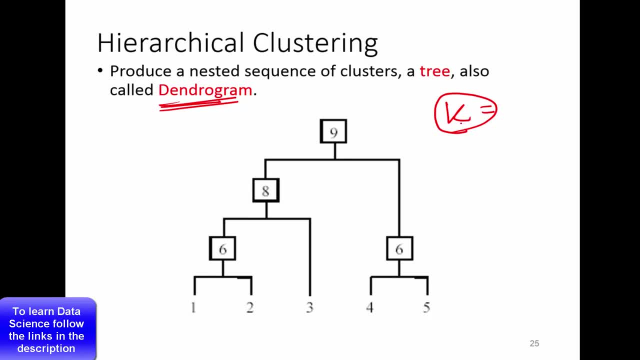 it in K-means. Rather, the clustering algorithm will provide help us understanding how many actual clusters are present in your data. So you need not know how many clusters are present a priori or before you use algorithm. So that's one. 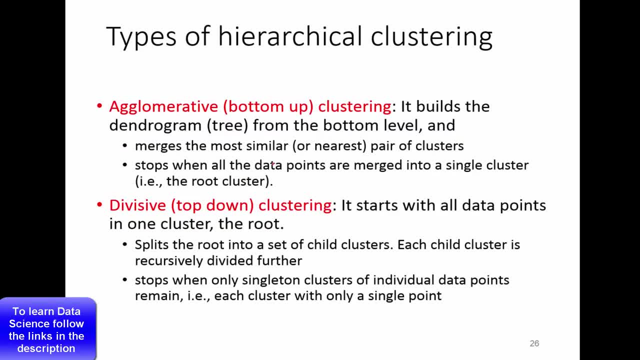 advantage over K-means. So there are two types of hierarchical clustering. One is agglomerative, which is also known as bottom-up clustering. It builds the dendrogram, the one that we saw in the last slide, from the bottom level. 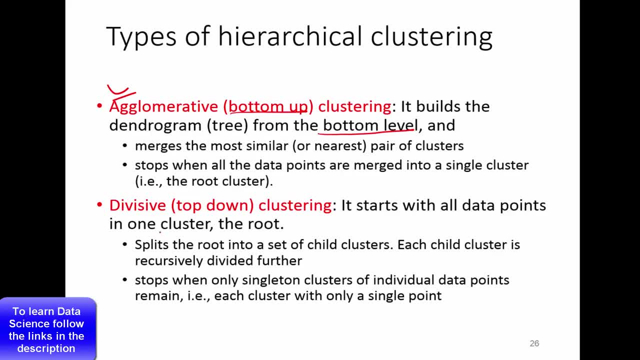 And we'll talk about it what it is. The second one is the divisive clustering, or top-down one. It starts with all data points with one cluster. So you know I'll talk about it how it's different. So that's very easy to understand. So in agglomerative clustering, 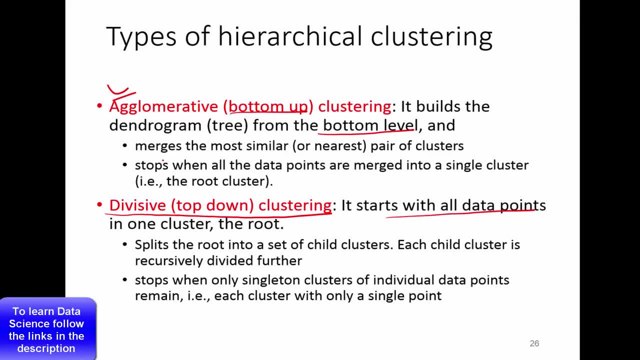 it builds the dendrogram from the bottom level and it merges the most similar pair of clusters. stops when all data points are merged into a single cluster. That means it merges the most similar pair of clusters. Let's say we have, you know. let's say there are 10 data. 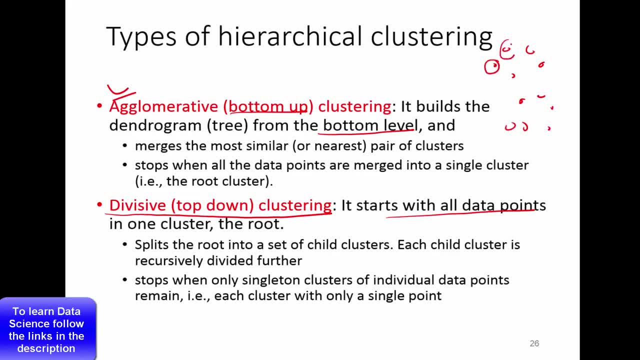 points. So it takes each data point as a cluster. So this is agglomerative clustering or the bottom-up clustering: each data point as a cluster. So if there are 10 data points, there are 10 cluster, 10 data points n cluster. That is iteration 1.. 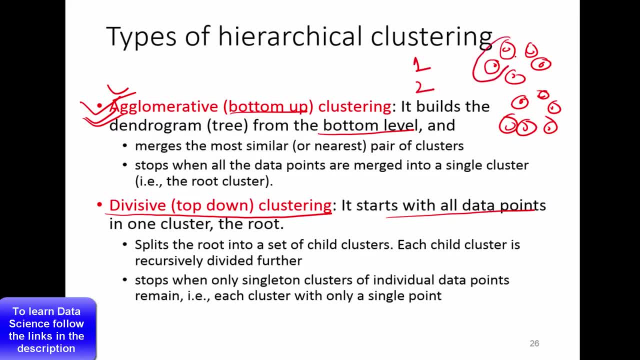 In the iteration 2,. it combines the next closest cluster. These are two closest. It combines and forms one cluster. These are two closest clusters. It combines and, you know, form another cluster. These are two clusters. It combines and forms another cluster. These two and these. 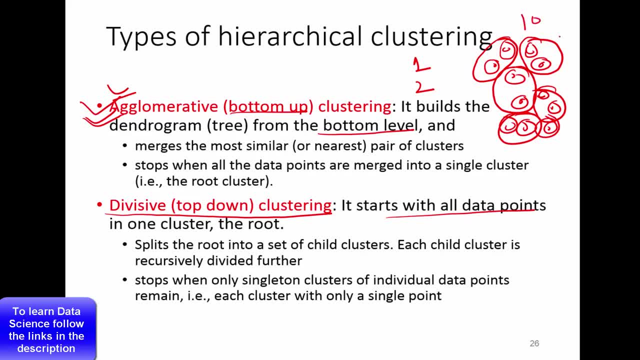 two and so on. So now, from 10 clusters, we have got 5.. From 5, we'll have 3, because 2, 2 and then 1 will be another cluster. From 3, we'll have how many 2.. From 2, we'll have. 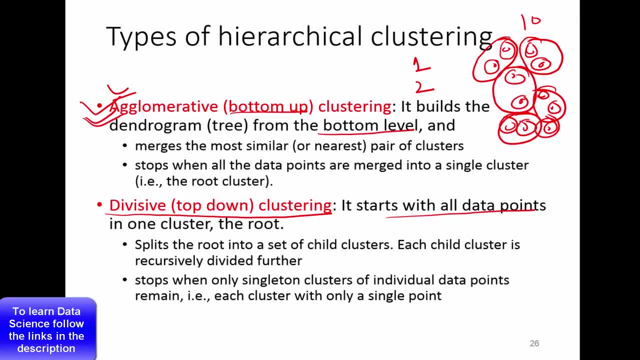 1.. So till the time you have that 1 plus 2., which combines all data points, this algorithm will run. so there's a fixed number of- uh, you know steps involved in this. unlike k means where you cannot calculate what is going to be the fixed. 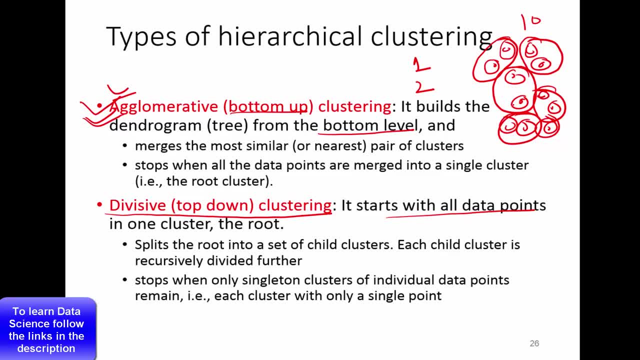 number of steps. here you can easily calculate what is going to be the fixed number of steps. it depends on what's the number of data points. right, depending on the number of data points, we'll be able to calculate this very easily. all right now. once we have this, we try to create a 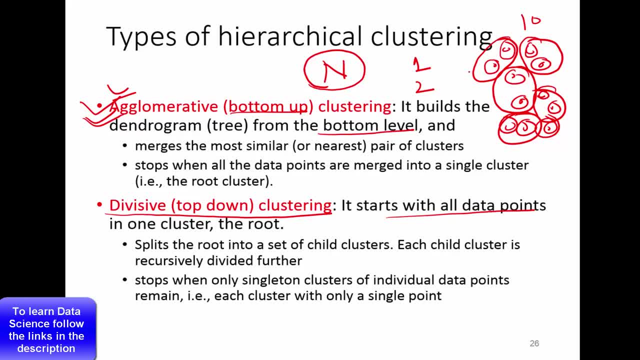 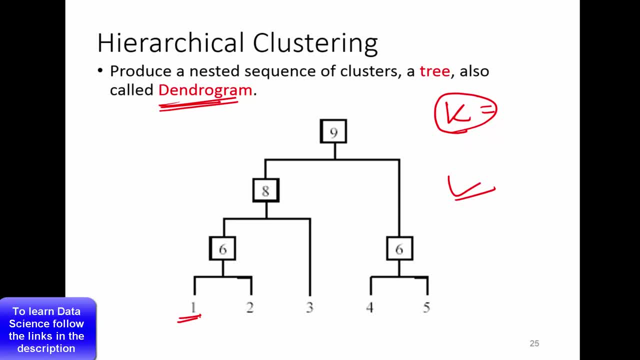 decision type. decision tree type. uh, you know graph that we just saw in the last slide, which is called a data graph. right, simple, right. the first observation is now taken as a one cluster. this is one cluster. this is one cluster. this is one cluster. now these two are closed, so we combine. 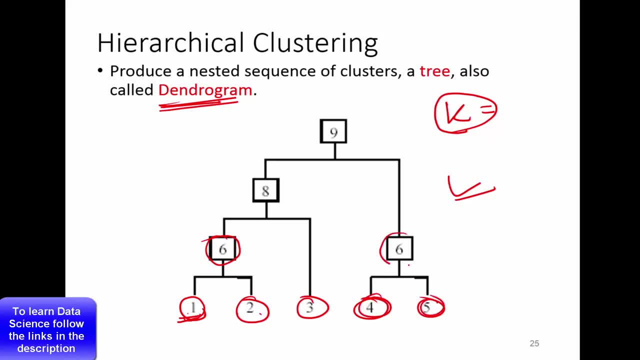 this one. this two are closed, so we combine two from this one. now, this one and this sixth and third have been combined from eight, whereas for six there is nothing. so eight and sixth have been clustered into nine. right, it's very easy, from bottom we are going up, so that's why i told 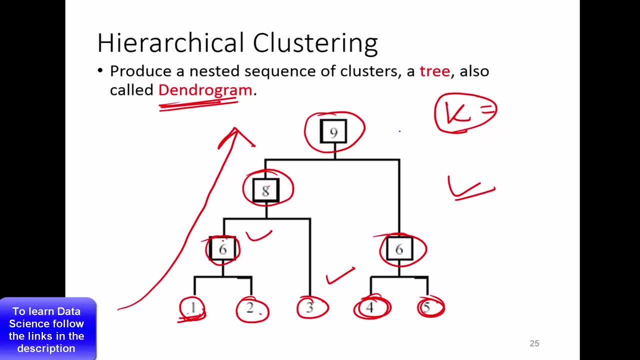 it's bottom up, and how many clusters do we have? well, we can take, you know, this entire segment to be one cluster and this entire segment to be one cluster, and we can take, you know, half of this whole segment to be one cluster and this entire segment to be one cluster. 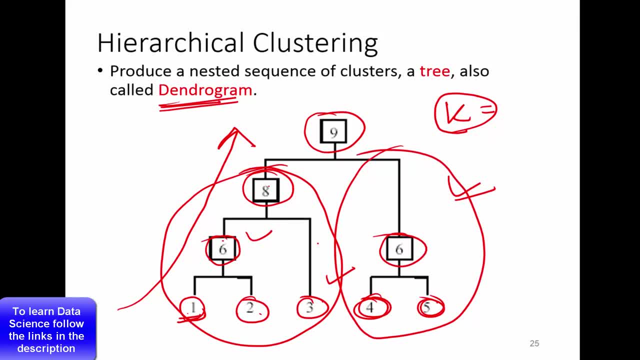 and how many clusters we have. uh, we will have to use the same detailing求. you knowέ, this is segment to be one cluster, two cluster. we can also have three clusters. we can take this one as one cluster, this one as second cluster and this one as third cluster, but depending on you know what. 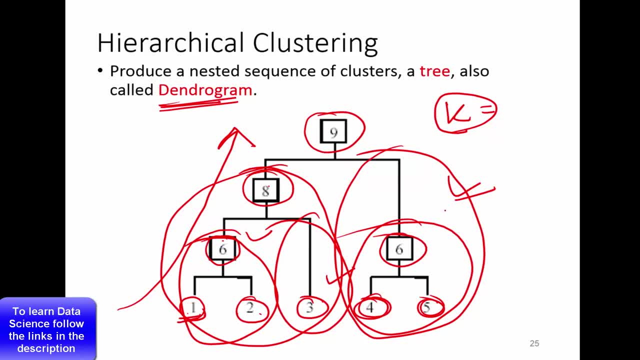 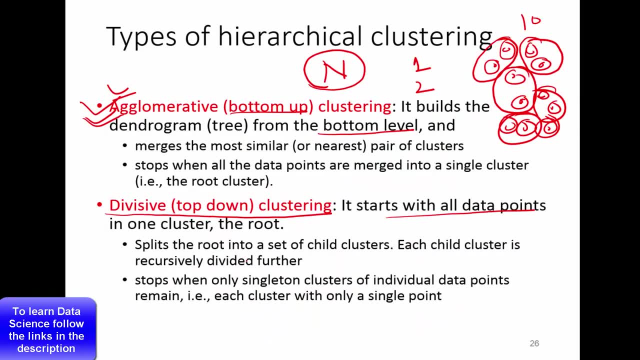 what is best suited for us. depending on our analysis, we'll be able to know what exactly is the number of clusters and you know which data points will improve each cluster. the top down is exactly opposite. you start with all data points and start breaking down into smaller, smaller. 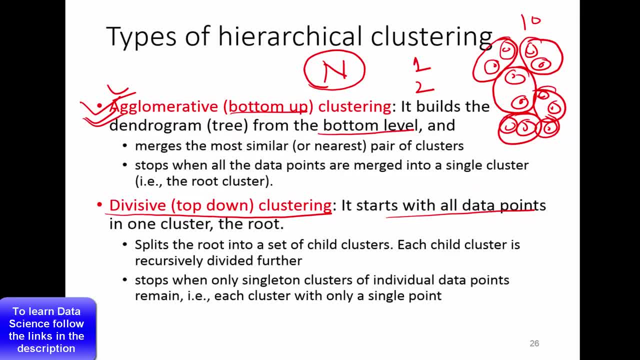 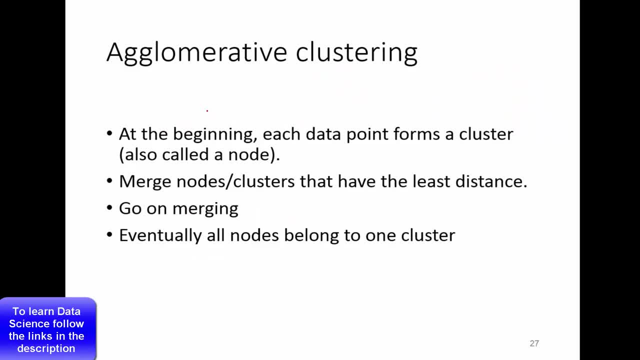 clusters till the time each data point is a separate cluster is exactly opposite of that. so whatever i have just demonstrated, it's just written in different points at the beginning. each data point forms a cluster, also called node merge nodes, a cluster that have the least distance. okay, 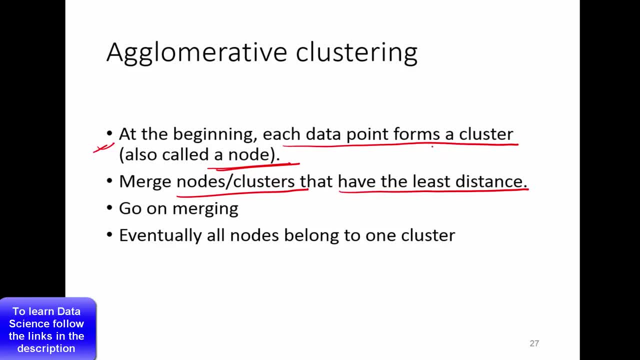 the closest distance, the closest clusters, you just merge them, okay, and you keep on merging in each iteration till the time you have just one cluster and then you form the dendrogram. okay, you just form the different steps how you kept on merging, okay, and then you decide how. 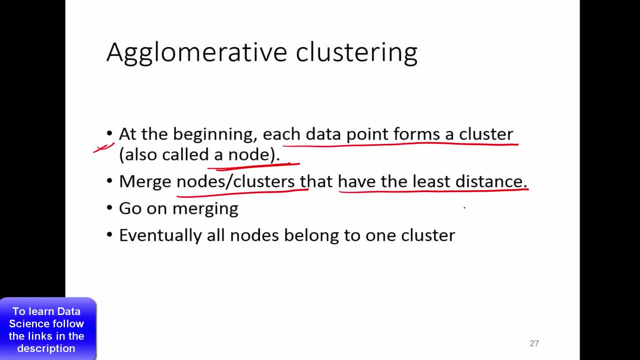 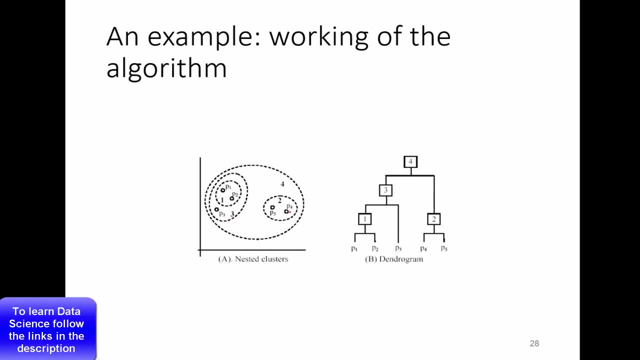 many clusters you want and when you decide that you can easily calculate, you can easily find out which observation belongs to this cluster. it's very easy, just by looking at the dendrogram. it's very clear. here is an example. okay, so there are how many? uh, well, there are five data points, okay, p1, p2. 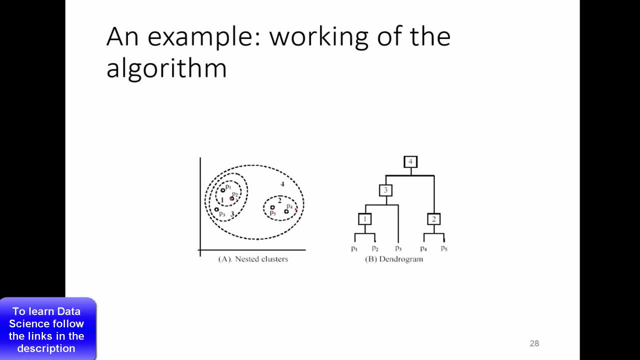 p3, p4 and p5. okay, the first step, uh, each p1, p2, p3, p4, p5. uh, with the cluster first step we had five cluster right: p1, p2, p4, p3, p4, p5. right then p1 and p2 are closed very close to each other, right the least distance we calculate. 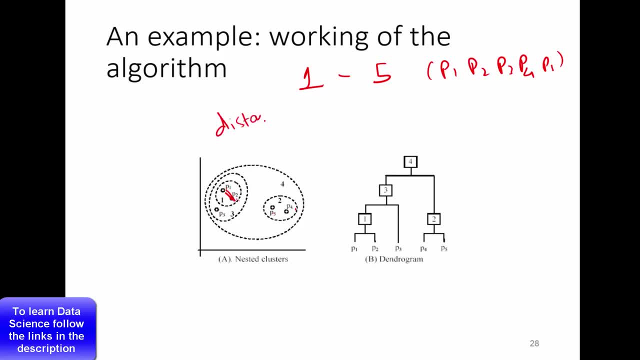 the distance. you know, every time in in cluster, we are calculating distance. hence we will study more about calculating distance. how do we do that? in the next few slides. so we calculate distance between p1 and p2. that's happened to. that happens to be the least, so we combine them into one. 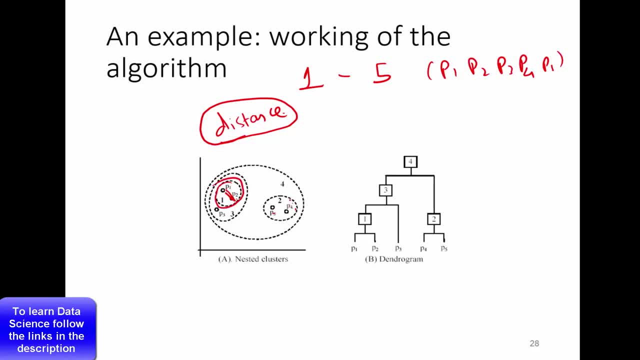 cluster. here also p4 and p5 are closed, so we combine them into one cluster. p3 remains alone, right? so there are now three. plus in second iteration we have three clusters: p1, p2 in one cluster, p4, p5 in another cluster and p3 in a separate cluster. so cluster one, cluster two and plus. 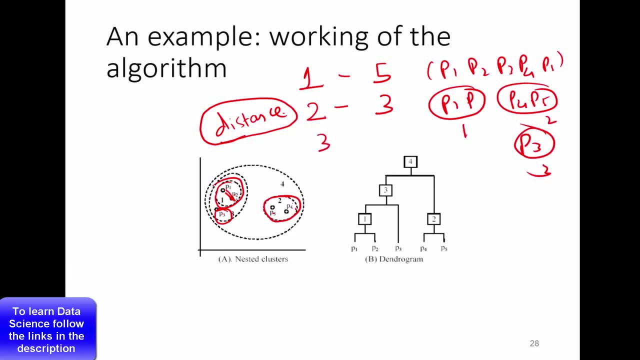 the feature three cluster, now in addition three, p1, p2 is cluster one, eight. so this cluster, cluster one and cluster three, are very close, right again they have been merged, so we merge now. so now we have two clusters. now we have two clusters, so we merge now. so now we have two clusters. 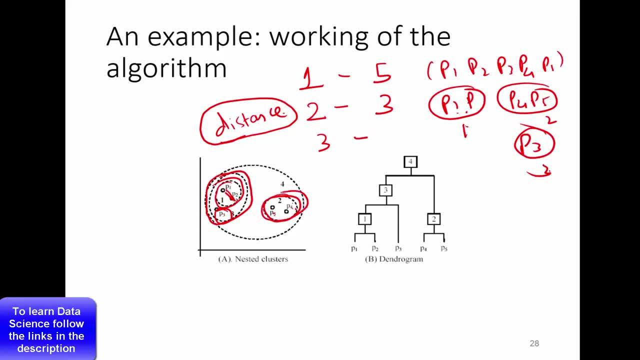 P4, P5, so this is one cluster. P1, P2, P3 in a single cluster, so two clusters, right? So these two have been merged, so we have P1, P2, P3 in one cluster and P4, P5 in another cluster. all right, 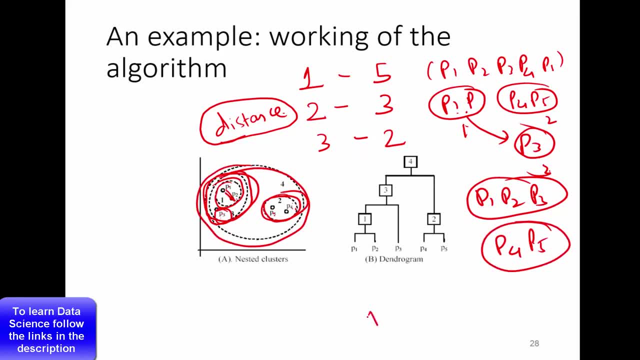 In the final stage we just combine everything. so we just have P1, P2, P3, P4, P5 in one single cluster. simple, right, The way you started, with each point to be a cluster and then started merging points to form, you know, a bigger cluster, and so on. 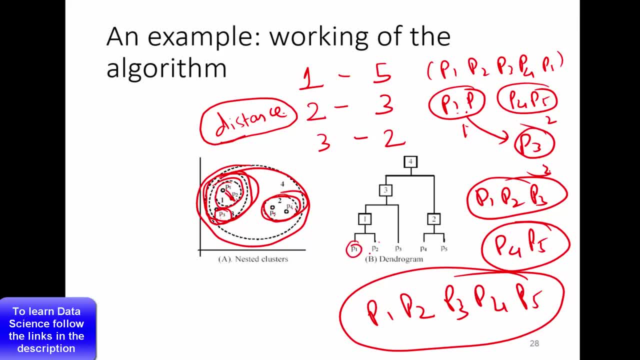 you just build similar diagrams right: P1, P2, separate cluster combine to form another cluster. P3, separate cluster combine with become this cluster here. P4, P5, combine to become cluster 2, cluster 2 and cluster 3 become cluster 4, simple. 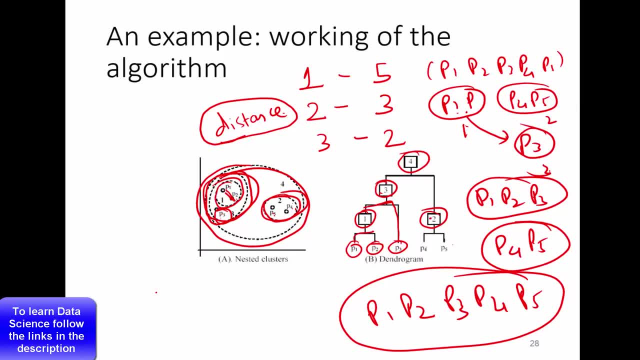 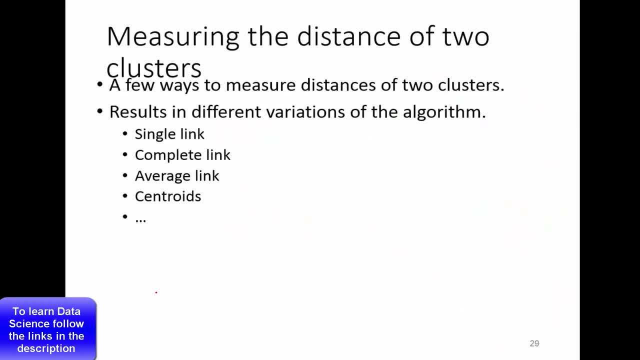 So, looking at the dendrogram, it gives a lot of good insight. We will know how many clusters do we want it finally? So measuring the distance is a big issue in clustering. We need to know how do we calculate distance, and there are many methods to do it. 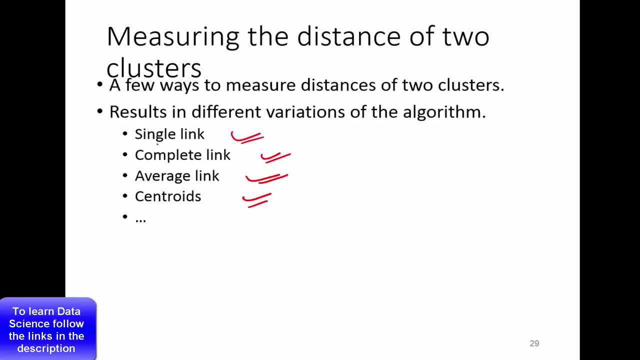 One is single link, complete link, average link, centroid. Well, let's go through as to how do we calculate distance between different points. So that's what matters to us. Whether it's k-means clustering, whether it's hierarchical clustering, we need to find out the distance in between the data points. 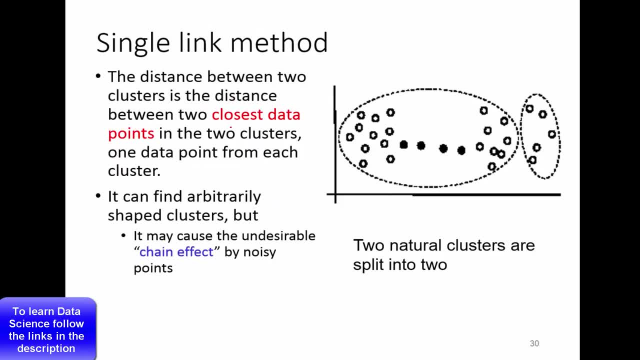 In single link method. the distance between two clusters is the distance between the closest data points. So here is cluster 1, this is the closest cluster 2.. The distance between these two clusters is the distance between the two closest data points. 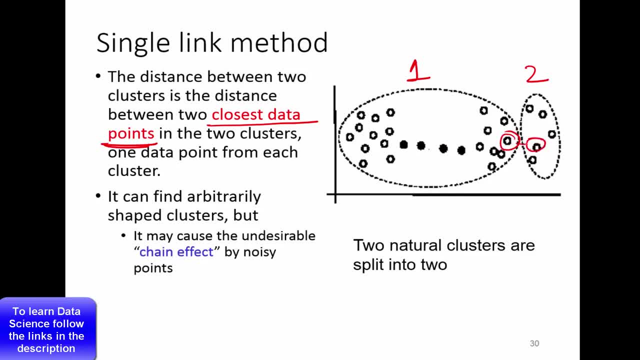 This is a data point and this is another data point. They are very close, right? So this data distance, let's say this is distance d. So d is the distance between cluster 1 and cluster 2, because these two points are very close. 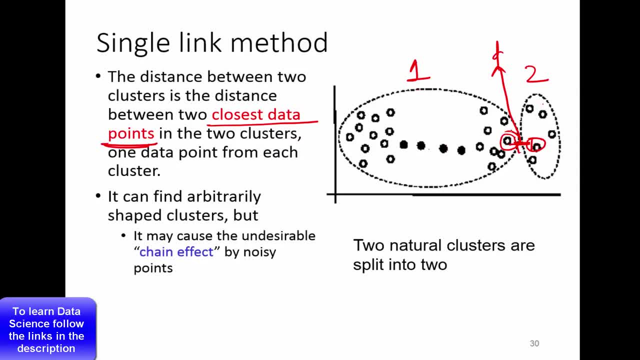 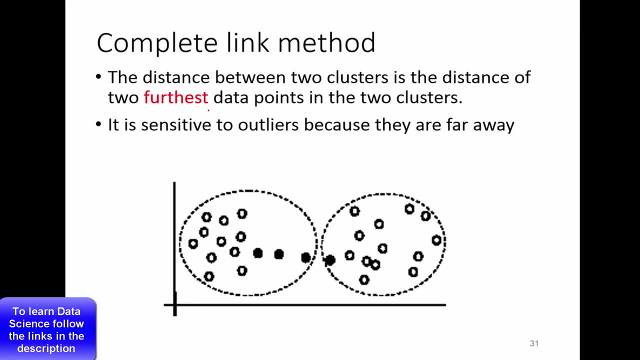 And whatever is the distance between these two points, we will consider that as the distance between these two respective clusters. Now, this is one way of calculating. The other one could be we will take exactly the opposite. So we will take the two files. 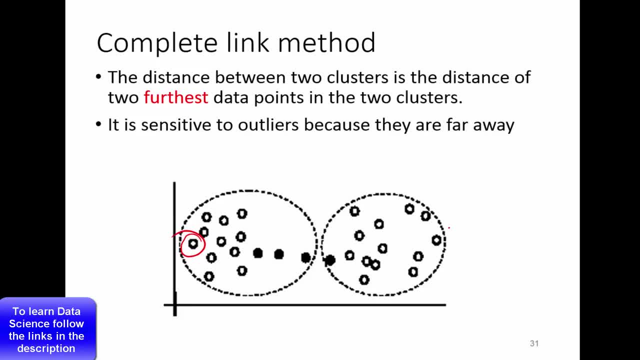 They are the farthest data points. So two farthest data points- one is here, the other one is here, right, They are the farthest to each other. So, whatever be the distance, we will call that as the distance between the two clusters, cluster 1 and cluster 2.. 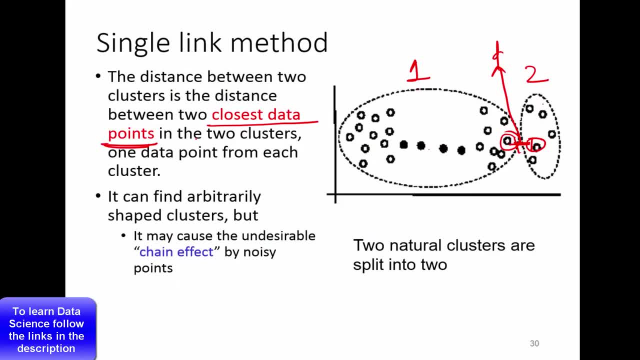 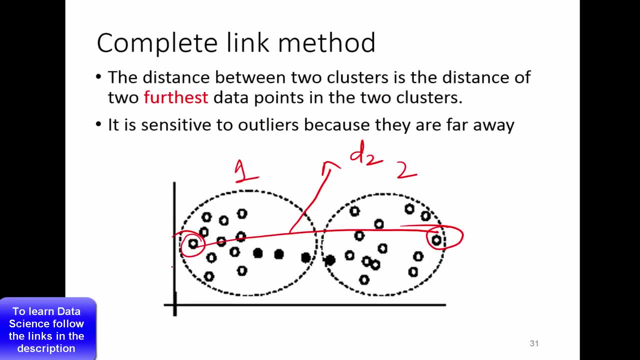 Now you can see the way you take the distance between two clusters. the clustering algorithm partition the data accordingly. You can see the whole lot of this data has been clustered into cluster 1. And a small section into cluster 2.. On the other hand, if you take complete link method, where you take the farthest data points to be the distance between two clusters, 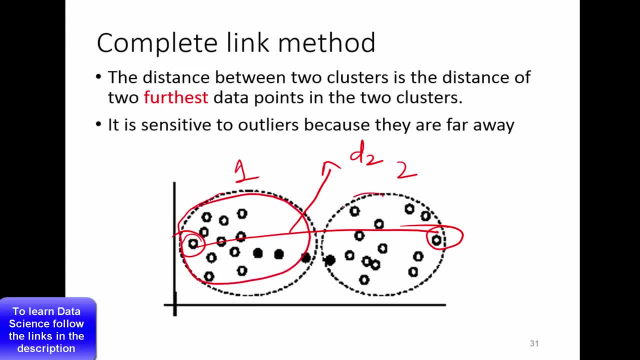 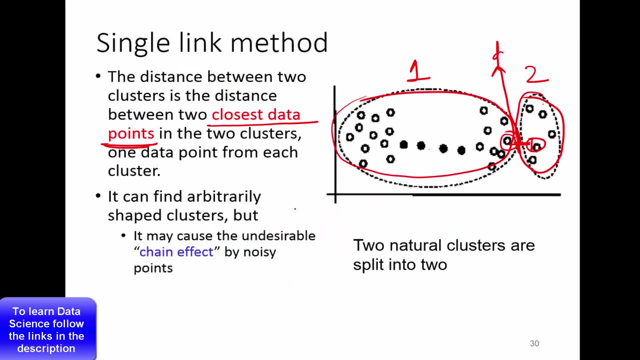 you see one set of clusters. data points are here. the other set is here, right, So that's somewhat different from what we have seen in the previous slide. So, depending on which method you know the algorithm is using to calculate the distance between two clusters, 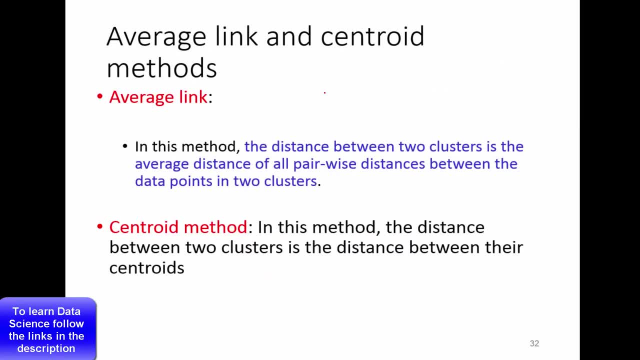 you will get different. Average link is just averaging it out Instead of taking the extreme points, whether it's closest or farthest, right Closest or, you know, farthest In average link you take. the distance between two clusters is the average distance of all pairwise distance. 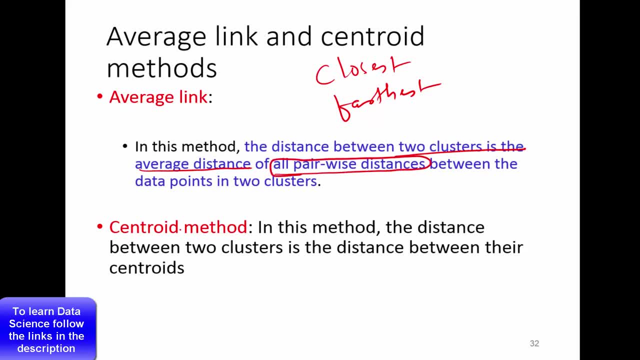 This is to be kept in mind. all pairwise distance okay between the data points in two clusters. You take each Data point in cluster 1, each data point in cluster 2, calculate pairwise distance for one data point. You take a distance for every other data point in the other cluster and for second data point. 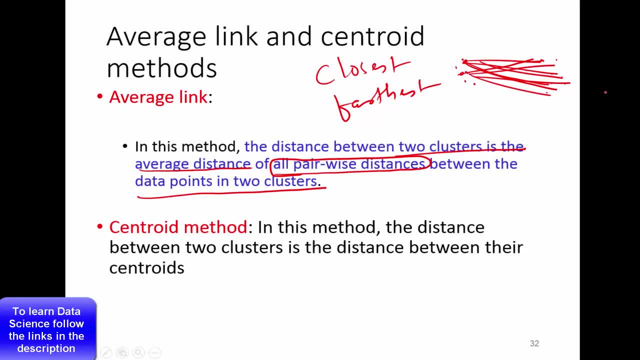 take distance for every other data point in the second cluster and you take the average of that. Whatever is that average, you take that as the distance Centroid method is that the distance between two clusters is just the distance between the centroid, which is very simple. 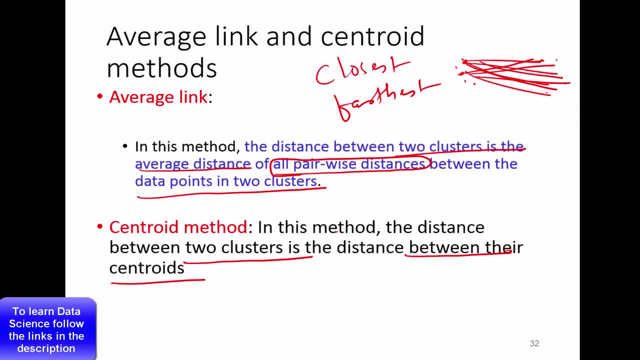 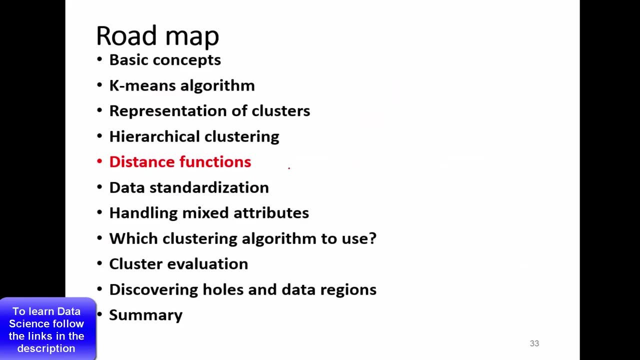 And easy to calculate and also quite easy to understand. You take the centroid of each cluster and whatever is the distance between these two cluster, two centroids of the respective cluster- is the distance of the cluster. All right, so we'll now talk a little more about the distance function. 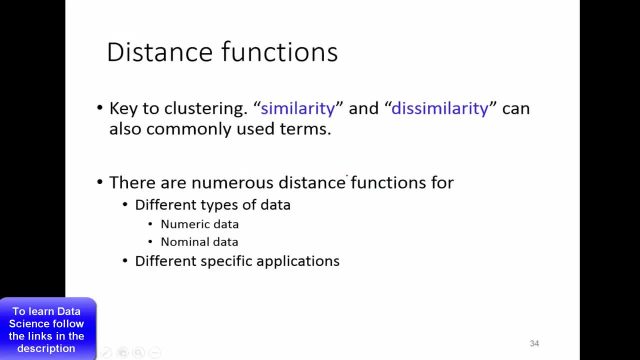 We'll then talk about data standardization. Well, the distance function is used to, you know. find out This Similarity and the dissimilarity. okay, we are interested in finding out similar observation which can be put into one cluster, dissimilar observation which can be put into a different cluster. 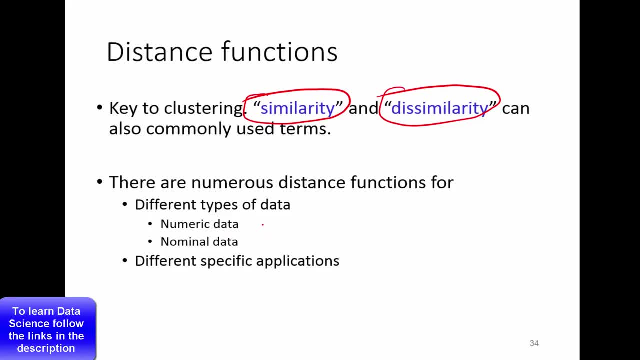 Now, there are different types of data you will receive. One could be numeric data, which is, you know, more of a continuous data. There could be nominal data, which could be more of a dummy form, or ordinal data, and so on. 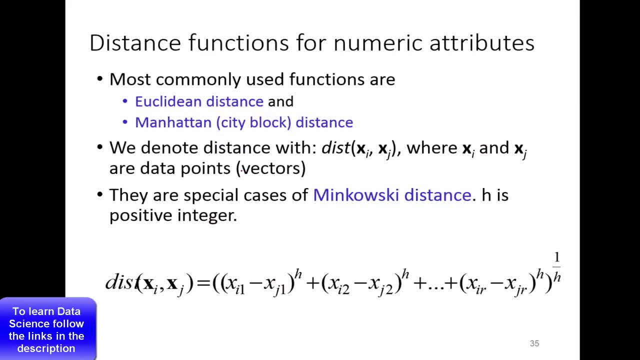 In such cases you'll have to have you know different types, Different way you can. you have to handle- I mean, the algorithm handles, of course You don't do it when you use the software, but the underlying algorithm will deal differently depending on the type of data. 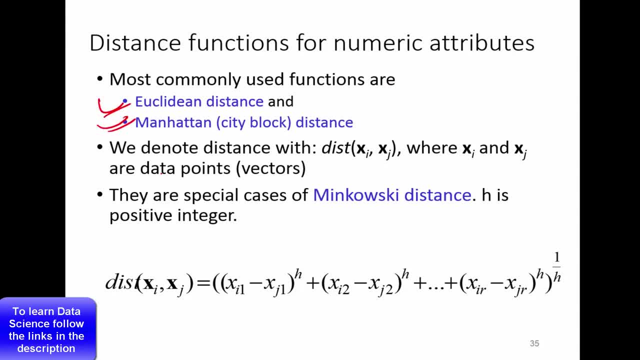 The most commonly used functions are: Euclidean distance, Manhattan distance. Okay, this is the generalized form of a distance formula calculations. The h can take any values right. So if it is h equal to 2. It is an Euclidean distance. 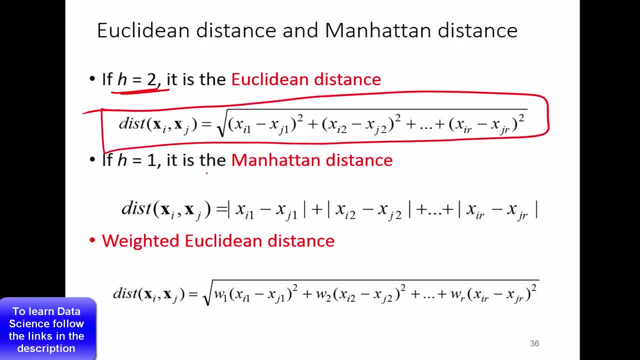 So this is an Euclidean distance of finding out distance. If it is equal to 1, then you get Manhattan distance. You take simply the modulus of the difference of the data points and take the sum Weighted. Euclidean distance is also possible if you want to give different weight to different observation while calculating distance. 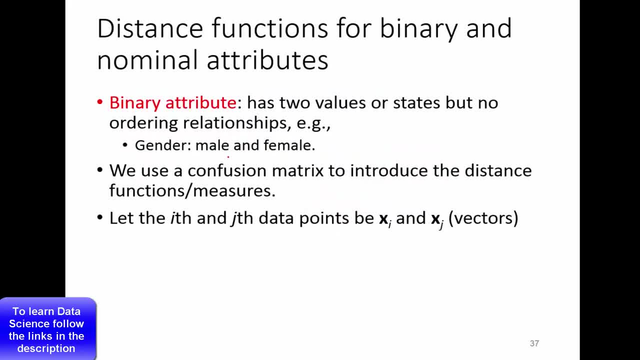 So that's also possible. Now you could also have binary attributes, Values, let's say 1 and 0. Some cases where you know you have values like 1 and 0. For example, let's say, male has been denoted as 1.. 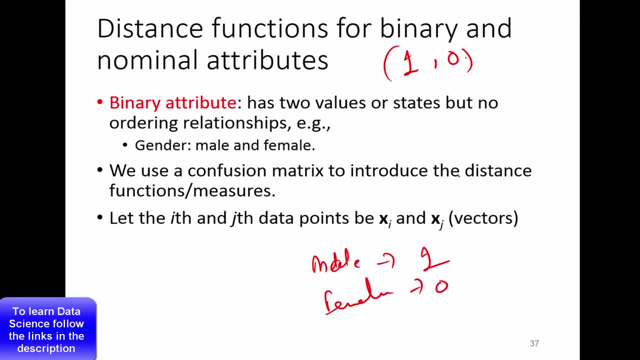 Female has been denoted as 0. So in that case, how do you calculate distance? Because distance makes sense in continuous data. but how about you know binary data or categorical data? So what we use is the confusion matrix. 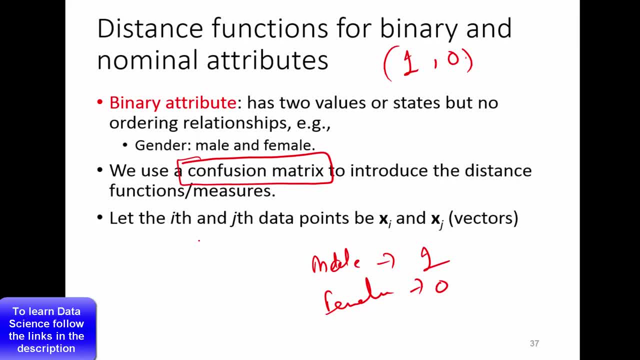 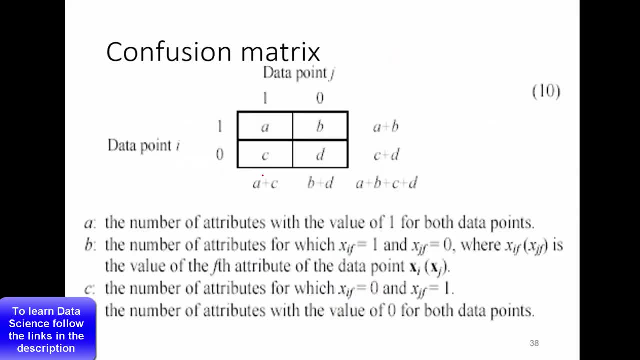 To calculate the distance. So how do you do that? You take the ith and jth data points. Let's say they are xi and xj, which are in vector form, by the way, because it has got different values. 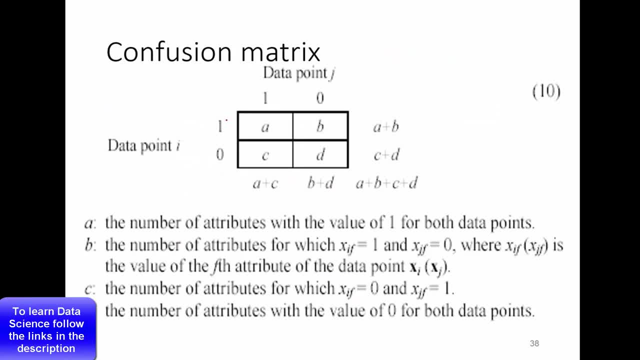 And then you calculate how many times you have xi taking a value of 1 and xj taking a value of 1.. And the number of times let's say is a: How many times xi is 1 and xj is 0?? 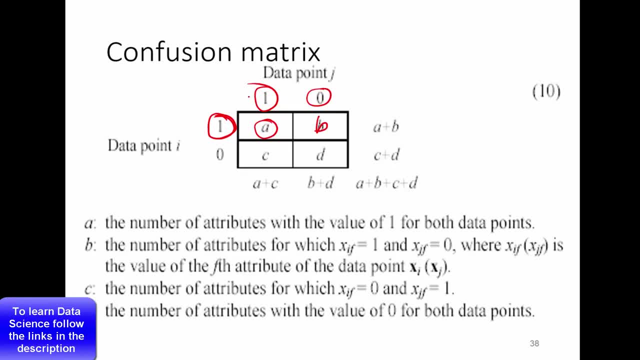 Number of times is b And how many times it is. xi is 1 and xi is 0 and xj is 1.. Number c: and when both are 0, it is number d. Now, when both are same, it is similarity, right. 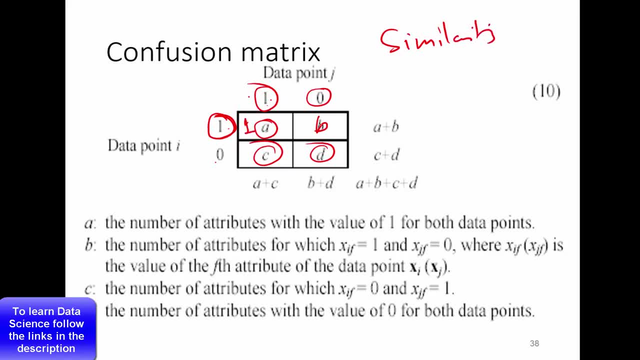 So the first matrix, so first this one and this one are the similarity When both are 1,, both are 0, which is a plus d. So this is similarity. b and c are when they are dissimilar. That means 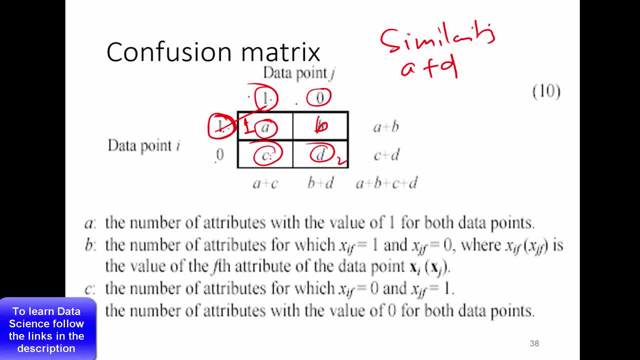 1 is like xi is 0 and x1 is 1 or x1 is 0, xi is 1 and xj is 0. So they are dissimilar, right? They are not similar. So that is dissimilarity. 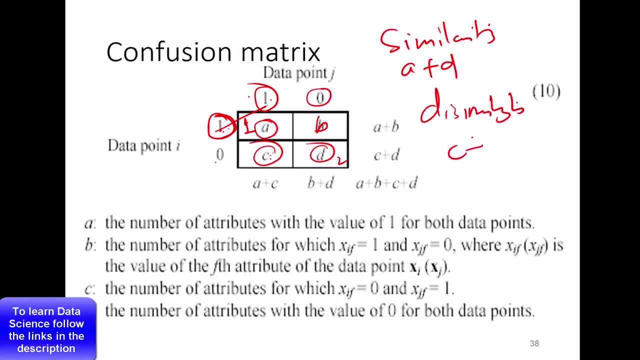 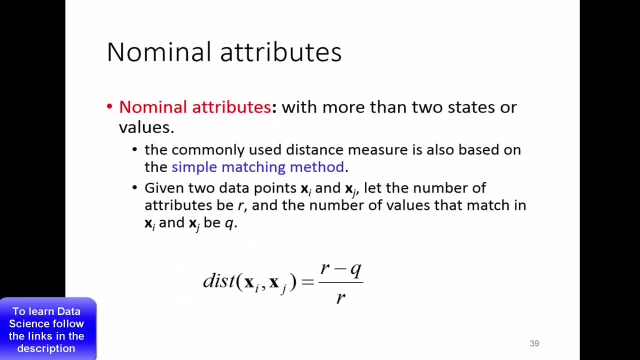 So dissimilarity is nothing but the distance. c plus b is the distance. So that's the way you calculate the distance between binary variables In nominal. If it is a nominal variable, that means it has got more than two categories. 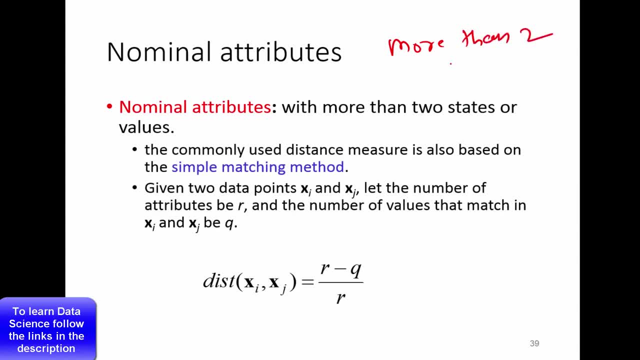 More than two categories, Two categories. In that case it's simple to calculate. It's just a more generalization. You take the total number of categories- Let's say that is the r- And you see wherever there is matching cases. 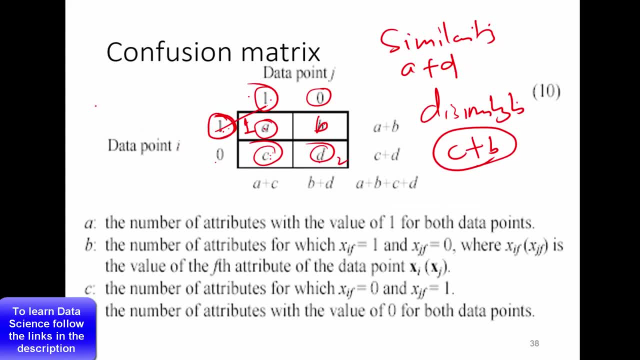 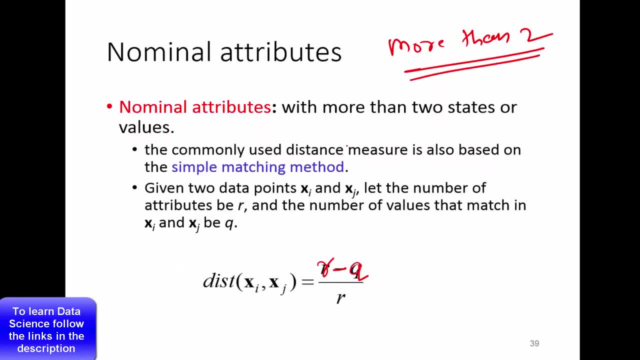 That means here you can see matching cases: right a plus d, a plus d. where they are similar, right Same. Both are 1, 1 or both are 0, 0.. Similarly, When you take various nominal values, let's q be the times where you know they are both the same. 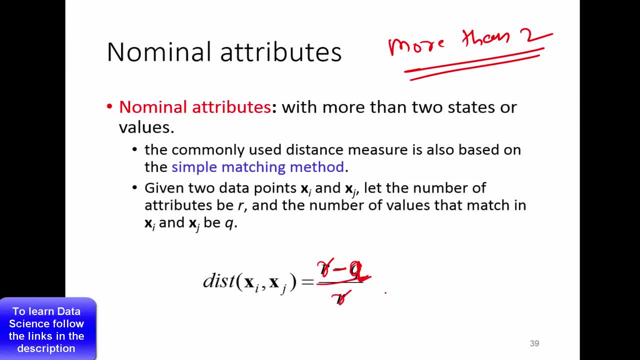 So take it out from the total number and divide it by the total r. So if r is the total number of you know, you know total number of categories minus total number of times when you know they are matching, and then divide by total number of categories. that's the distance. 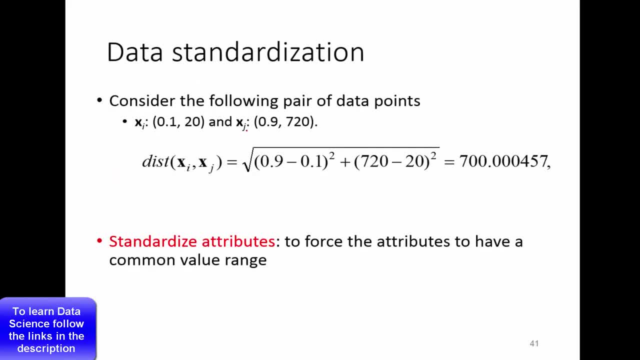 Data standardization. It's important. So how do we do data standardization? Why it's important? Now consider the following pair of data points and we'll see what's wrong with the way if we use raw data in plus d. 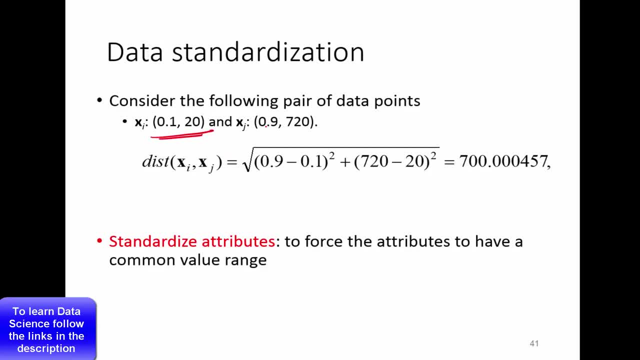 So here is xi, which is 0.1 and 20, and xj, which is 0.9 and 720.. The distance is 0.9 minus 0.1 square 720 minus 20.. So that's the Euclidean distance, and we find it out to be 720.. 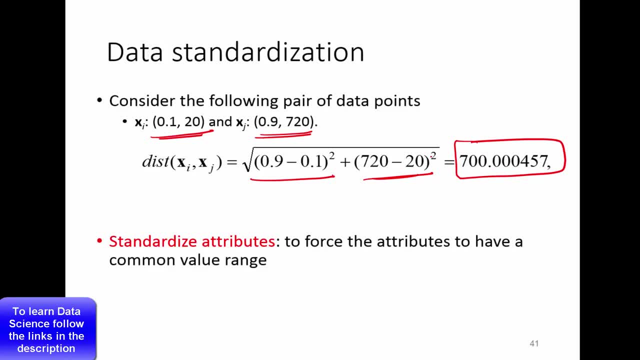 So that's the distance. Now you can see that the 700 that we have found out the distance is majorly because of this second term. right, The first term doesn't contribute much. That means it seems to be a biased thing, right?